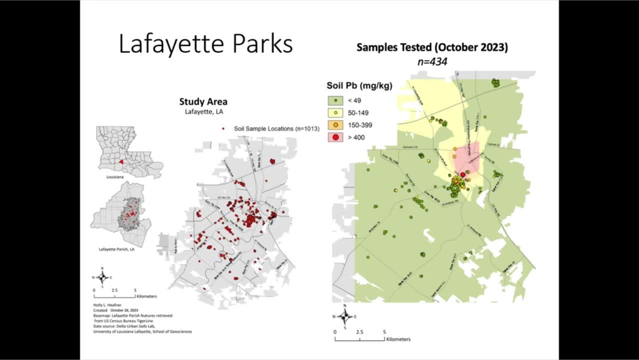 leaders to talk to their members and let us in into their properties, And I ended up going to some of the neighborhood meetings talking to residents and we get really great feedback from people. They want to know what's in their soil. They don't think about heavy metals. 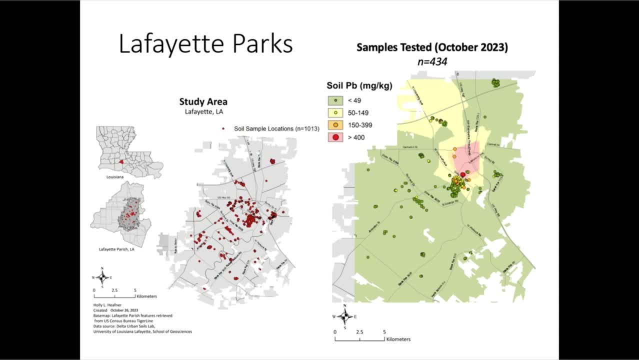 And we even were published recently in a local newspaper and in the channel interview on local TV channel, Dr Mielke-Mielke-Mielke, who is a member of the community of Lafayette. who is a member of the community of Lafayette. 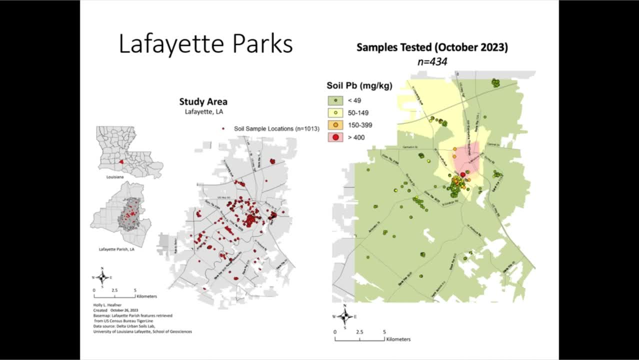 Dr Mielke-Mielke-Mielke, who is a member of the community of Lafayette, To bring more attention to this issue and get more samples from people. So for those who work with communities, it's a great way to do this is to reach out to local governments and work with them. 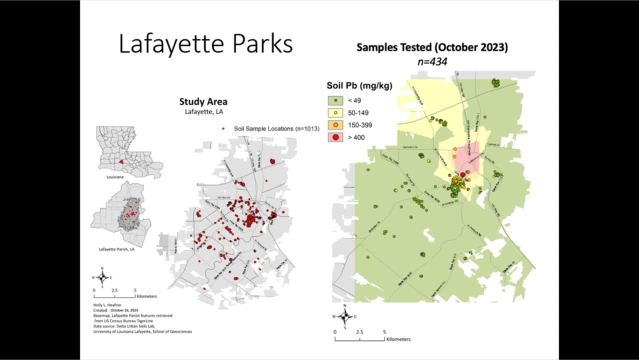 And of course we get a lot of help from USDA NRCS. So for this particular project, I asked Holly to pick just parks and get an idea what we would get concentrations-wise for heavy metals. Dr Mielke-Mielke-Mielke, we will have multiple heavy metal data and we will calculate. 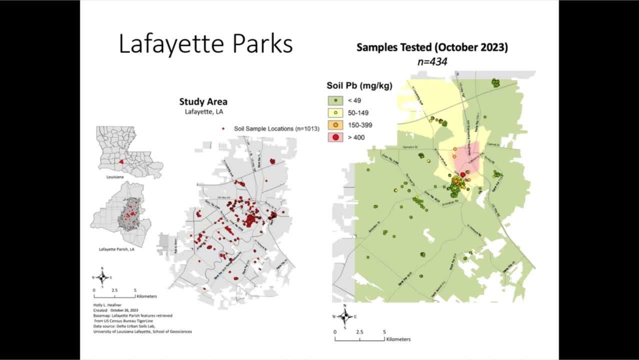 in the pollution indexes, Dr Mielke-Mielke-Mielke, but for this presentation just picked lead And you can see that again. inner city, when looking at the lead, concentration is higher in the downtown area, center area. 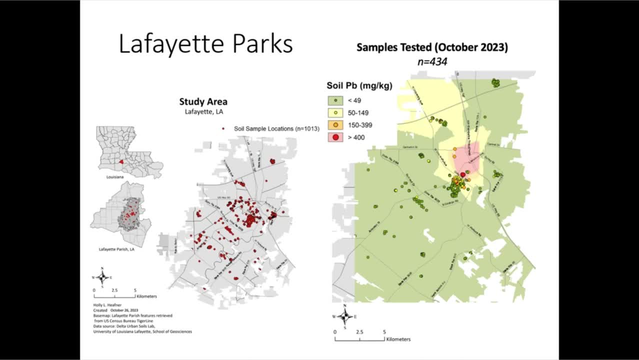 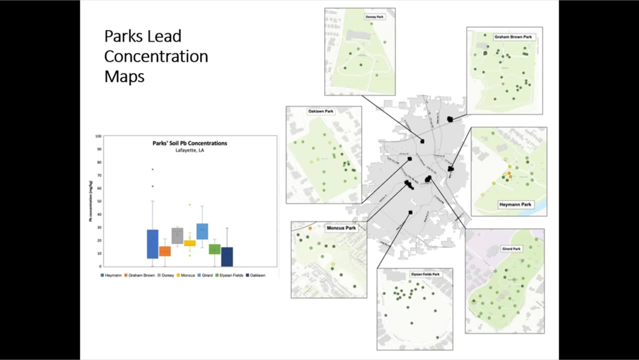 it's more historical and it disperses as we go further, with less people. So this measured lead in multiple sample, multiple metals, but lead in particular, in five different parks, 200 samples. What we found? that concentration you can see is very low. This is the Y axis. here is a hundred. 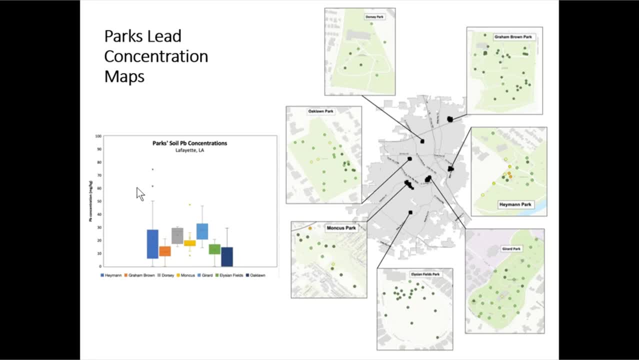 parts per million. Dr Mielke-Mielke-Mielke and only a couple of the outliers were here. Most of the samples are way below 50 parts per million. They were, on average, about 20 ppm for lead, which is natural background, which is great. 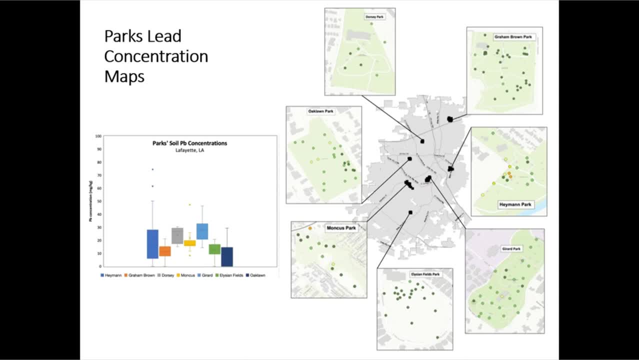 because in Louisiana they do a lot of festivals and all these parks are engaged in huge festival activities. People constantly have concerts, eat, having picnics there, So it's really important to test parks and see what we get. So, in terms of lead, it was great. In terms of arsenic, 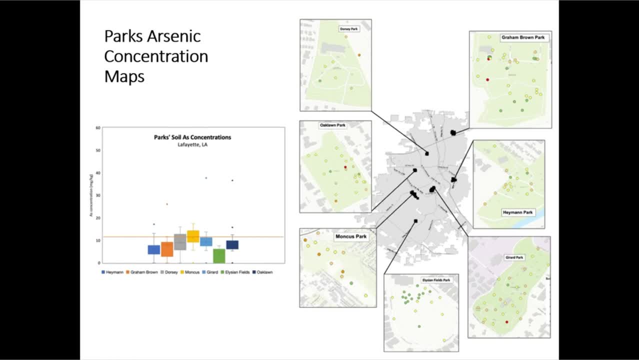 we saw some high concentrations, about higher than 12 ppm, which is Louisiana guideline. But arsenic is also naturally found in Louisiana soils because it's a sediment that's brought down by Mississippi. So it's likely this arsenic is not due to contamination but transport by sediment. 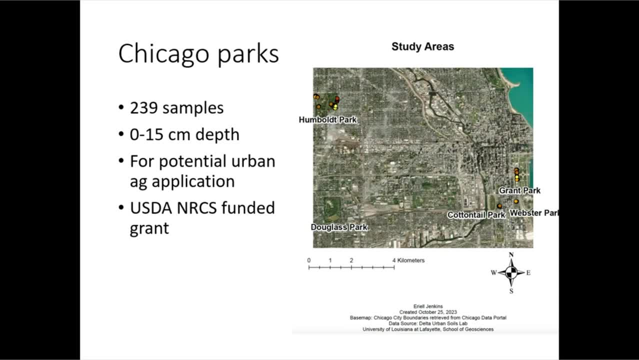 So in the Chicago parks. this is a quite interesting sample. We will continue talking with James Montgomery, who promised to help on this and figure out the solution, What we can do with these areas and these parks. So this summer we went to Chicago to collect. 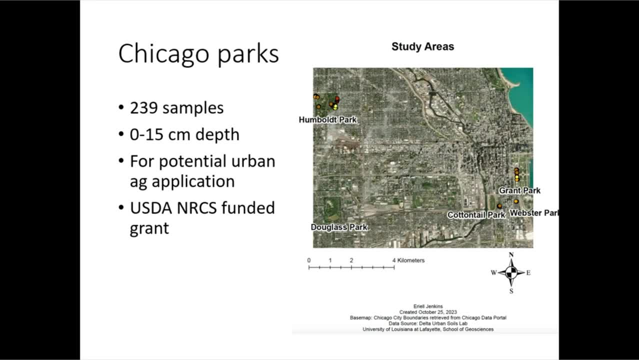 samples because we had the grant from USDA to analyze samples from two different cities. We will do Chicago and next one will be St Louis in collaboration with local NRCS. So we went to five parks and it was an interesting experience For my students. 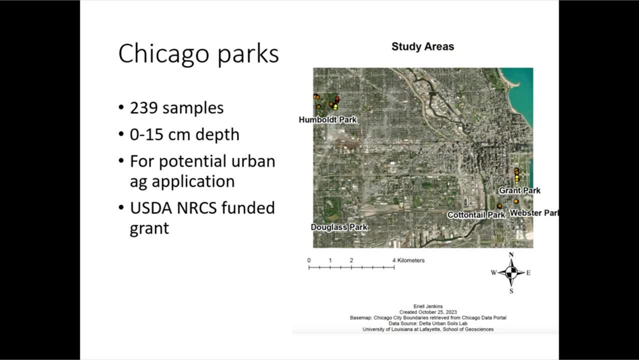 it was the first time flying on a plane and we had to take Ubers everywhere and with lots of bags and carry all the samples. So people gave us looks like what are you doing? And a lot of people approach us in the parks like what are you doing. But everything was great. We had multiple samples. 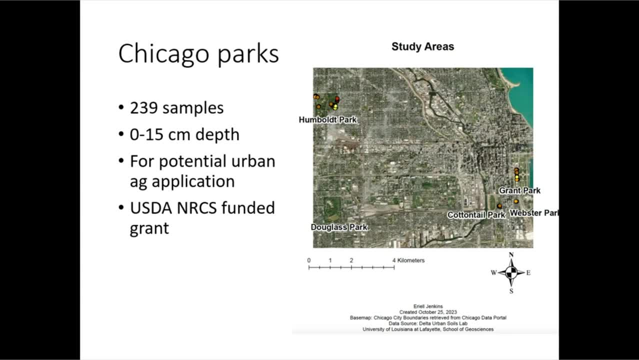 from very large parks like Humboldt Park or Grand Park to a small park. So we kind of wanted to see the distribution between different scale of parks. Of course Chicago has a huge, huge, huge park system and the city itself is really big. So we'll contribute to the existing soil survey and perhaps 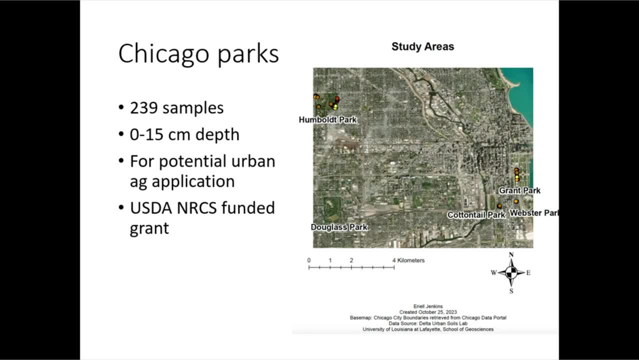 project that he mentioned earlier, So we can be part of larger database and see what results we're getting. But the idea for this particular project was to see if these parks can be used potentially for urban agriculture purposes And in some areas, like in Grand Park, we did see some urban ag sites. 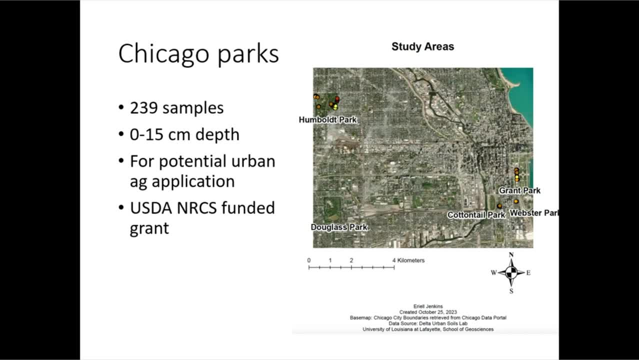 and it was really great to see the sustainable practices. They were doing mulch. It was really beautifully decorated and people were growing some collards. So I think we need to more of this, but we need to make sure its soil is not contaminated And we collected soils in the 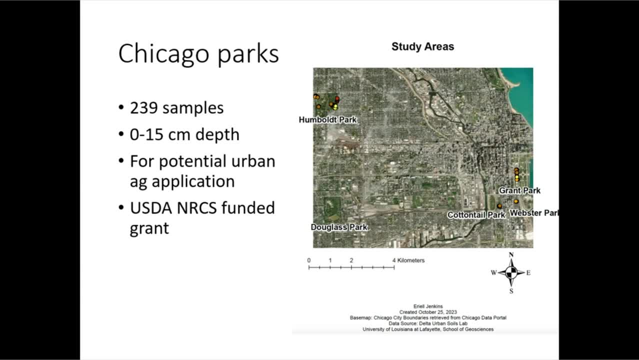 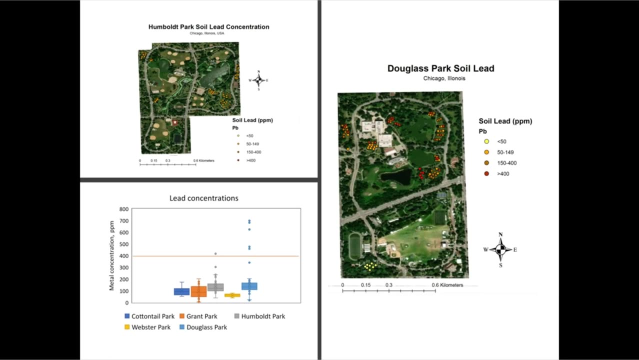 top soil 15 centimeters, So it was more work a little bit than do it at sample in Lafayette, because it was June in Chicago and it's super dry soils So but we had some fun. So what did we found? I'll just highlight a couple of maps to show you how the sites we 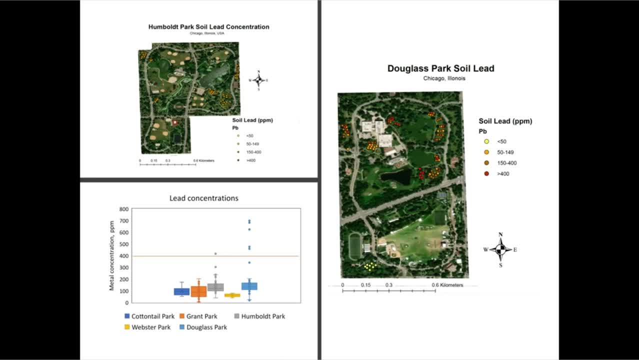 picked. We picked the sites in these five different parks I have here to show you From particular areas of the park that we thought could be used for agriculture, because not every open space in the park can be used for ag, because it can be a baseball field. Maybe it's a place. 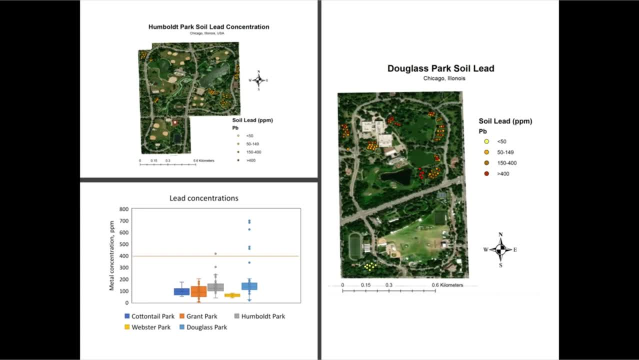 area for cafe or it's in the hill or something else. So this area that we choose we're looking like it was sunny enough, not many trees and a flat area that could be used for gardening, and here concentrations were more interesting. We see clearly that concentration in Chicago parks. 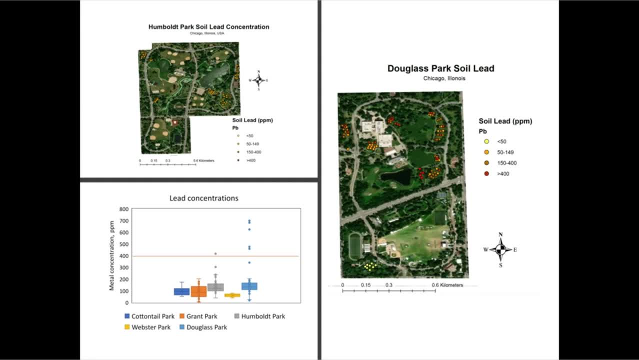 are much higher than in the rest of the country. So the concentration was higher than in the rest of the country. So this area was much higher for land compared to Lafayette samples. There were some of them. We had several outliers in Douglas park, more than 400 parts per million, which is the EPA. 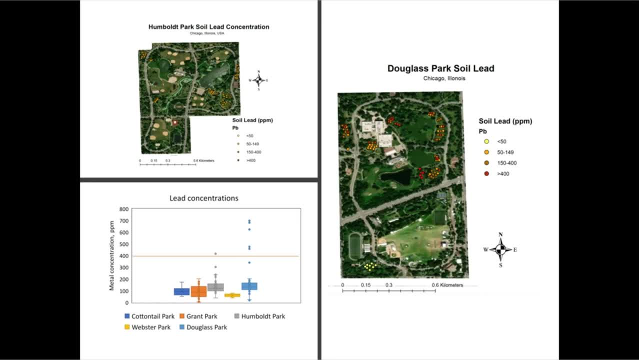 guideline for children playing in a bare soil. But most of soils exceeded more than a hundred parts per million of lead, So you can see some of the piers more like yellow, orange colors. but, Douglas, there's some quite a few of dark spots, more than 400 parts per million. But what's also interesting, to do to increase the use of arboreal sawdust or canola or other similar products that we can use with the farm. In particular, we are looking at the проcriation of Lavalier for the agrarian soil that we have found in the granite, which is the most common natural soil that we can find in the 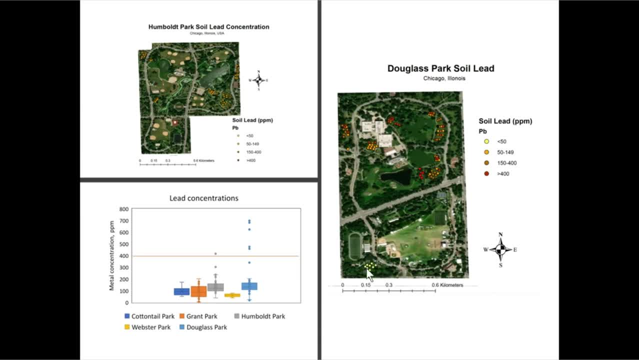 What we see in these parks is the heterogeneity. One corner here is less than 50 parts per million and the other side is a much higher concentration. So even in one park we see this heterogeneity because there are lots of, I guess, influences. 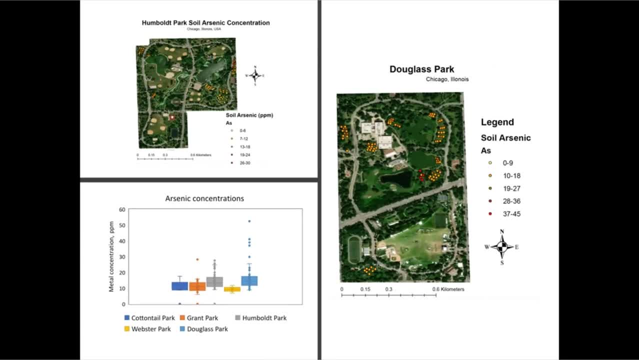 from the facilities that are around And arsenic. this was quite interesting to correlate. there are some areas where we could see both lead and arsenic higher. Douglas Park again had much higher concentration And last night I looked up the guideline for arsenic in Illinois and if anyone knows, what is arsenic concentration guideline? I found it 75 for Illinois So I wanted to put the line here, but I was like I better confirm this. someone in the know. In Louisiana it's 12.. In New York it's 16.. 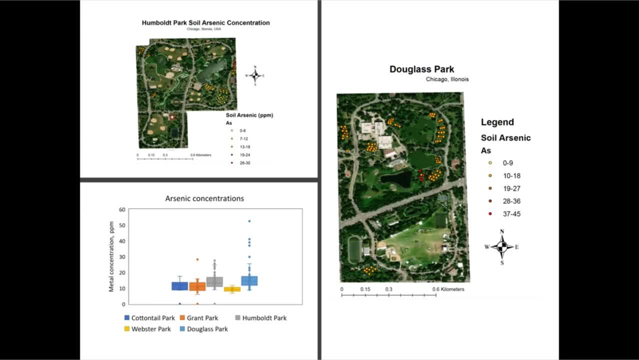 So, yeah, it's super high and, yeah, each state has its own guideline. If we consider 12 ppm as a guideline, You can envision here the line. that again a lot of samples, And it's a question of where this arsenic is coming from. 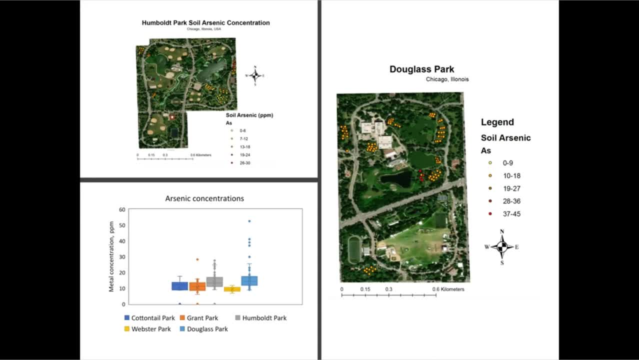 So maybe some of you know work in Chicago. we were researching last night and potentially maybe it came from the sediment or maybe there's some use with lead arsenate, because seems like especially in Douglas Park also they have lead and arsenic concentration. 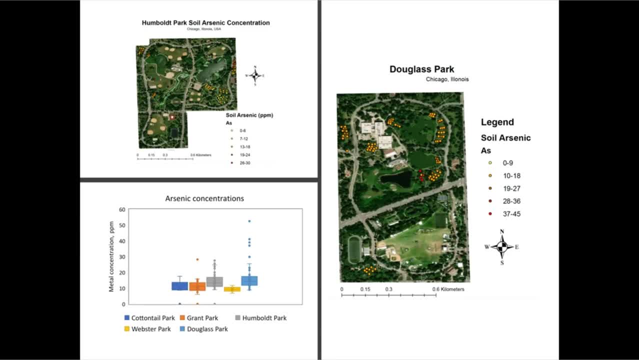 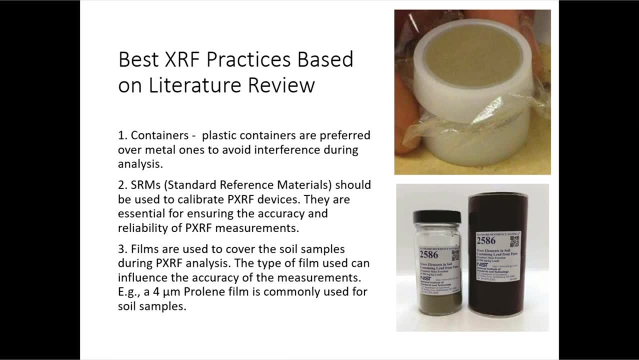 So this is something we're going to investigate more And again, it's a preliminary result, Since we talk about XRF, We're going to talk about XRF, We're going to talk about XRF. We analyzed the samples, we brought them, collected them in Chicago, collected in Lafayette. 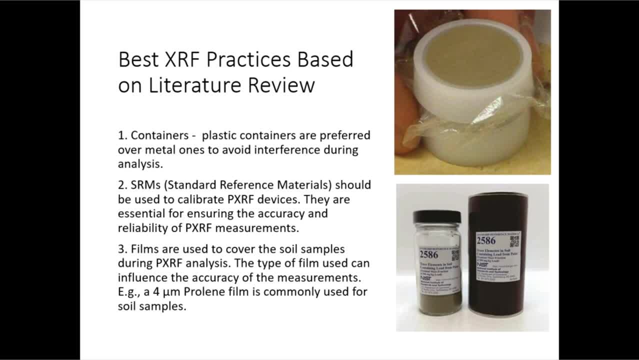 and analyzed them in the lab. We know that PXRF can be used in the field- demonstrated during our trip and workshop yesterday- but I wanted to highlight some best practices. if you're doing it in the lab, Anyone is using XRF, Okay. 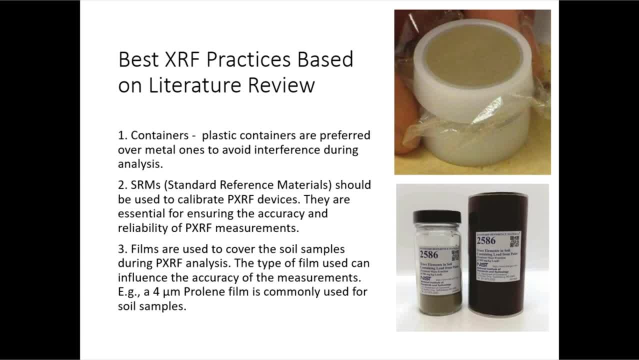 A few of you. So, for those who are going to use it in the near future, think of the best practices you can use to increase your accuracy of the results. Think of containers that you're using. We can measure heavy metals in soil in plug bags, but the best way is to use this XRF. 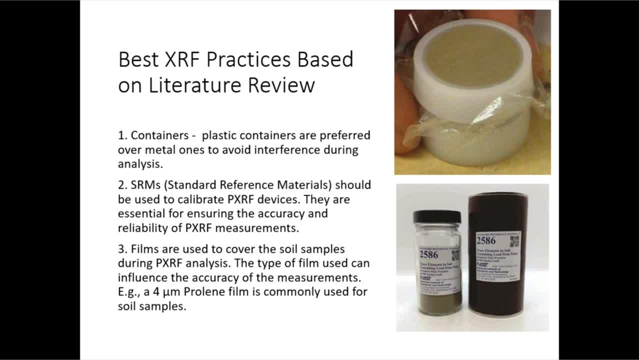 cups with the XRF film. This film is the best one, It's a four micro. there's proline film and it's commonly used because it has no impurities in it, So it's developed specifically for these measurements. Z plug bags may contain some impurities in it, but it depends on what grade of research. 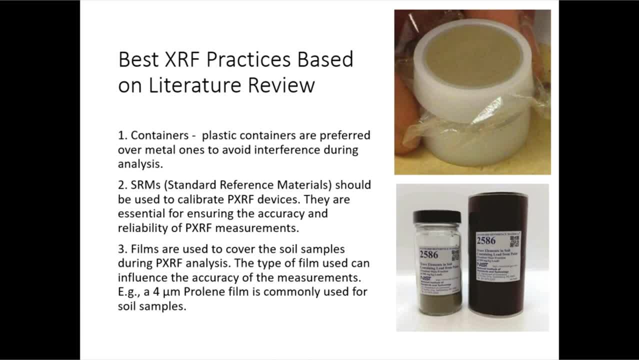 you want to do it. If it's for screening purposes, Z plugs are fine, But if you do something more accurate, more precise results, you should use the film. Use plastic containers. They're better than metal ones and better than Z plug bags. 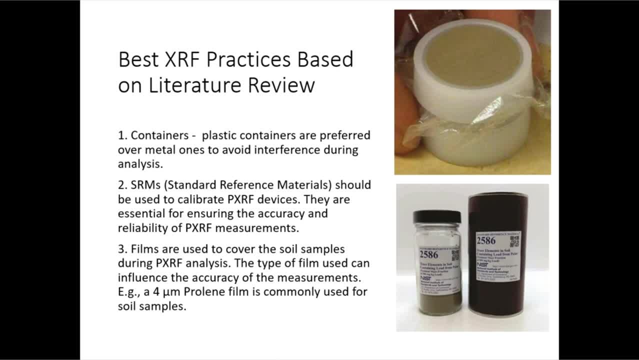 Use standard reference materials. This is just example of one, but there are multiple ones. It depends on what you're doing: sediment, soil or maybe plant tissues. There are multiple standards you can buy to build your external calibration curve. XRF typically have a calibration that's already installed in an analyzer itself, but you 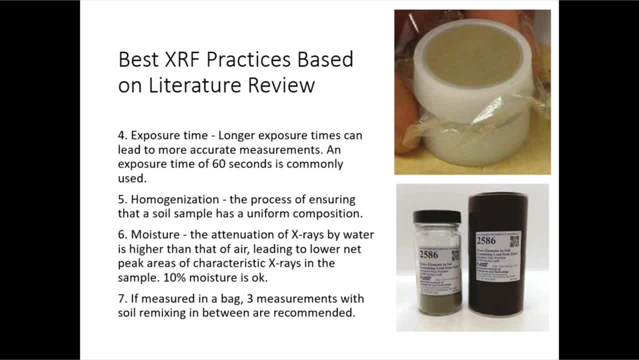 can use your own external standards. Then you want to think about exposure time. How long are you measuring your sample for? Found in literature that's at least 60 seconds. In my labs we always did 90 seconds. No difference. after 90 seconds, what to do? 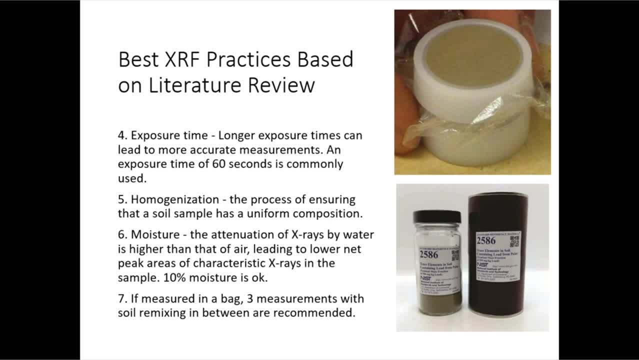 So 60 to 90 seconds is a good. Samples should be homogenized. If there's some pore space or grass, That's fine, Or gravel or pieces of branches or plants, it will disturb the readings. XRF sample needs to be at least one centimeter, but it penetrates only about two millimeters. 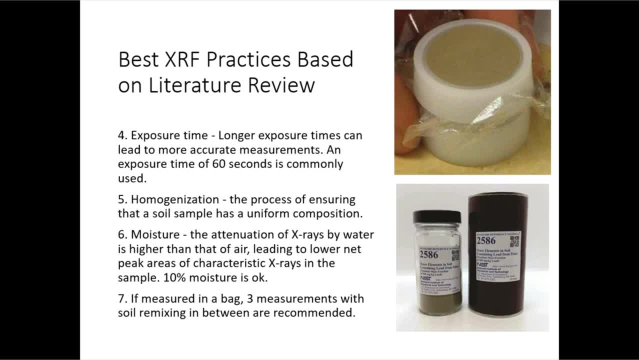 So the sample needs to, and it's about one centimeter in radius, like minus, So you need to make sure that surface is clean. Moisture is problematic if you have more than 10% moisture in the sample. That's why it's important to at least air dry the sample, but we typically oven dry. 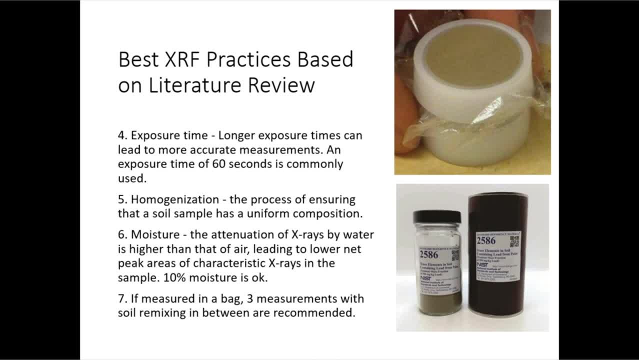 the sample for 20 minutes. So if you have 24 hours, 105 degrees Celsius, we sieve it. We crush it and sieve it under two millimeters and then analyze ref cups or maybe like small plastic bags, But we test them to make sure there's no impurities. 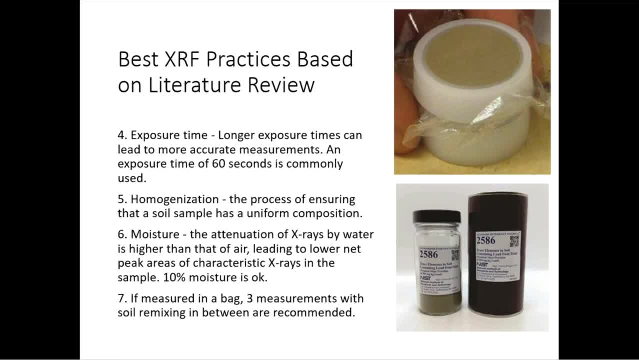 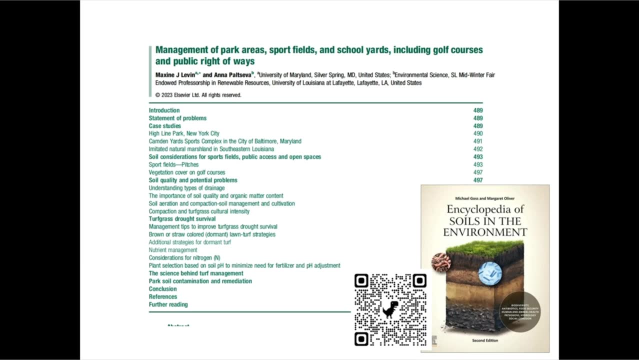 And if you do measure samples in bag, especially if it's in the field or in the workshop, do it two, three times to get an average, because each side will have a different concentration. So get an average. So we Actually, Maxine, published the paper that I encourage you to use your QR code and, if you don't want, 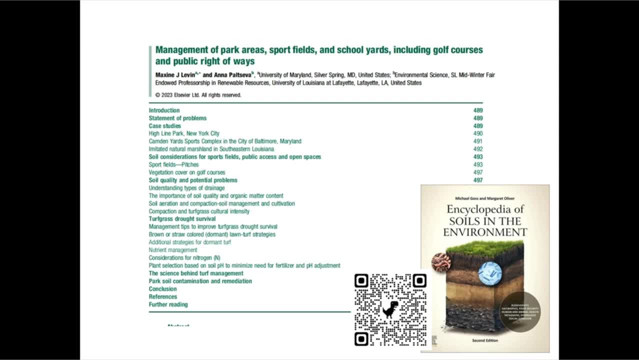 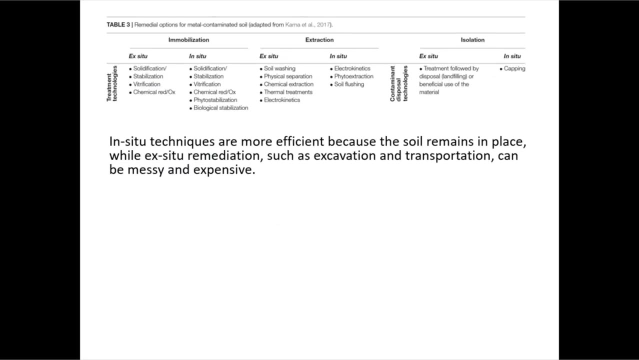 to buy it. you can email me and I will send you a copy. But this is a really great resource for management of parks, sport fields and schoolyards And it combines the best management practice with some current examples from urban environments. If we find contamination, what can we do? 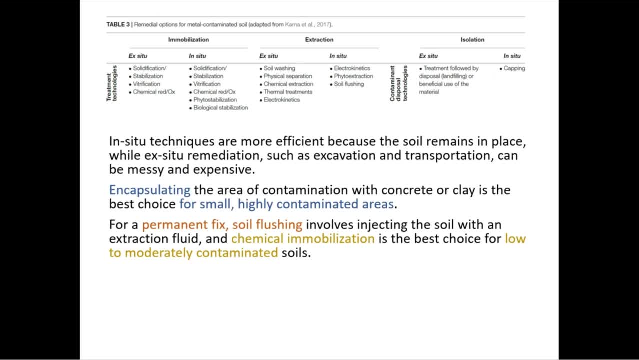 There are multiple ways and some of them were presented and will be talked later, But overall we have in situ and ex situ techniques that we use. So we have a lot of information. We have a lot of information, We have a lot of technical techniques that we can use to change the chemistry of contaminants. 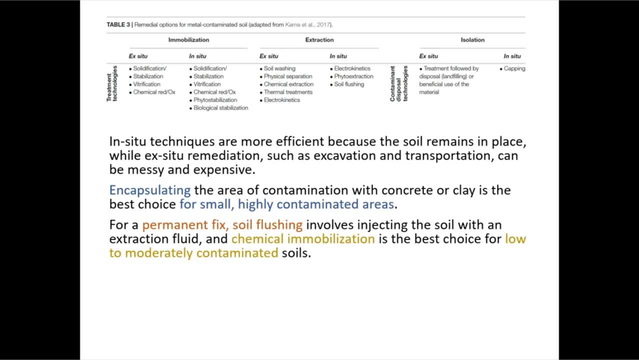 We can encapsulate it. if the contamination is very high, We can use the soil flushing. if To inject extraction fluids into the soil, we can use the different immobilizers to aid this contaminants. We can use phytoremediation, as someone previously offered to trees for jacket joiner. 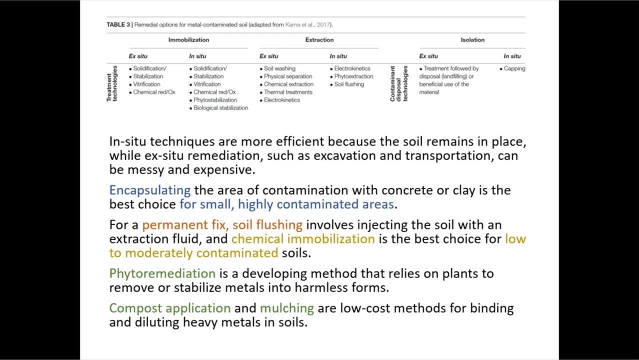 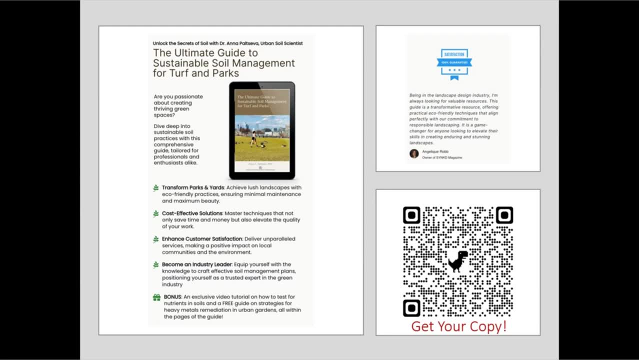 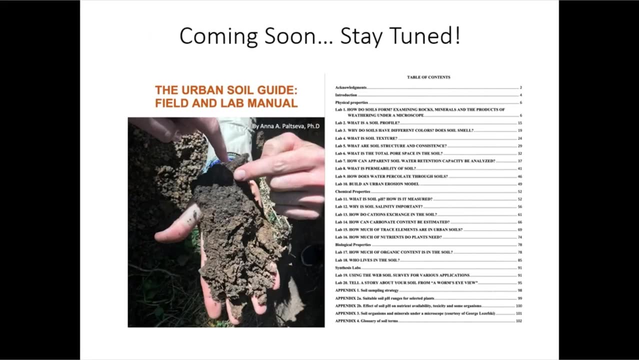 And, of course, we can use compost and mulch. There's something anyone can do. If you don't want to read that big, big paper, I have another guide that I recently created for sustainable soil management, So you can also use your code to download, And I want to brag to you that I'm publishing. 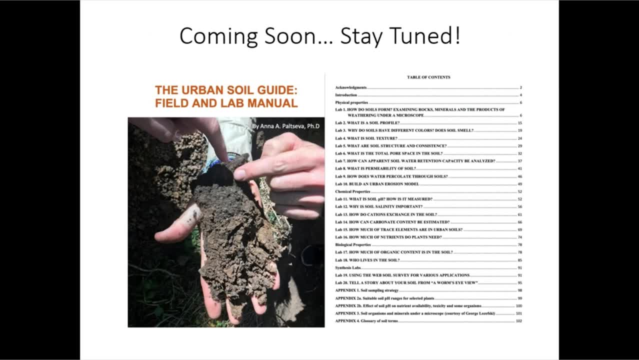 my urban soil guide and it's coming out in the early next year, published by Springer. So in the importance of networking it came from here. Springer reached out to me last year- triple essay meeting- And I said: if I have anything else I want to publish with